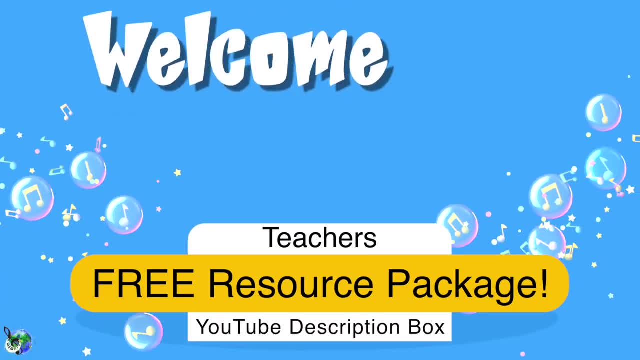 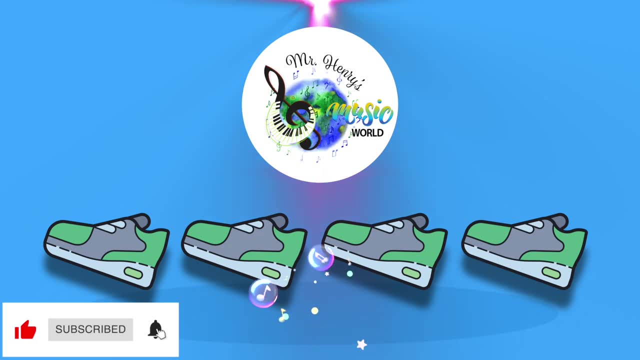 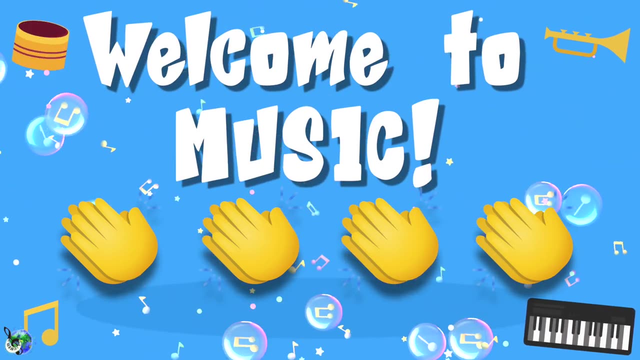 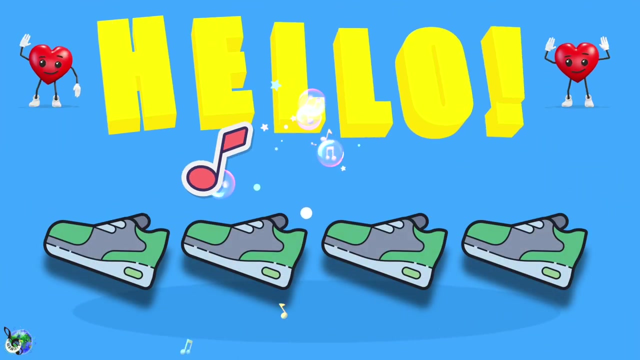 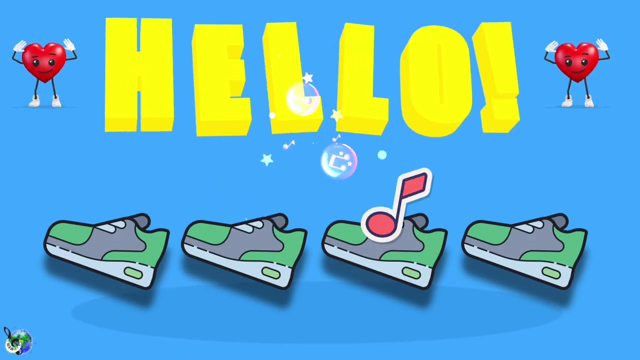 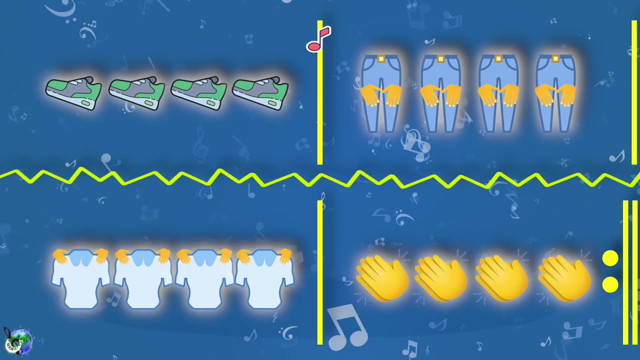 Hello, welcome to music. Hey, welcome back to music. Don't ever exclude it. It really is a true gift. So let's commit to learning about the elements. Work hard, cause music is too legit to quit. We have beat, meter, rhythm and pitch- The foundation of music. this is gonna be a cinch. 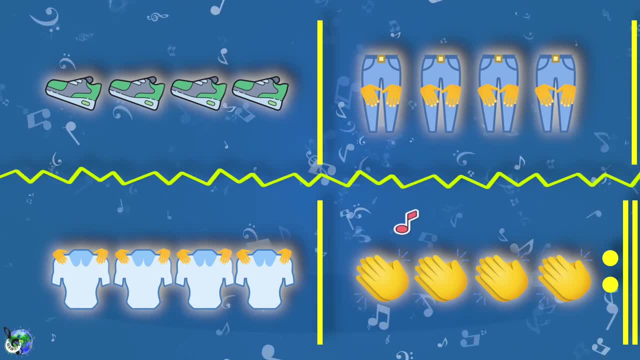 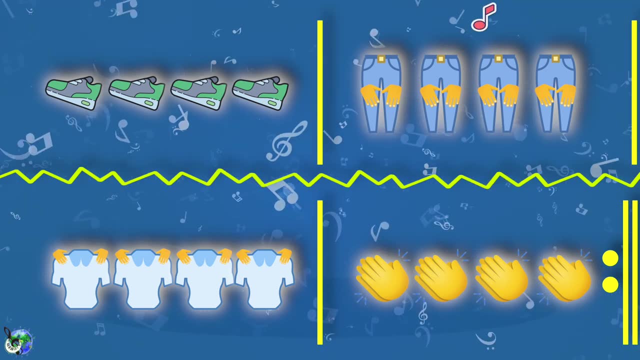 On to melody, dynamics, form, tempo and timbre, Hammer time, nailing down all the great manners that we need to make our music class great: Be respectful, responsible and safe. And don't forget awesome attitudes all around. Come on, y'all, we're moving. 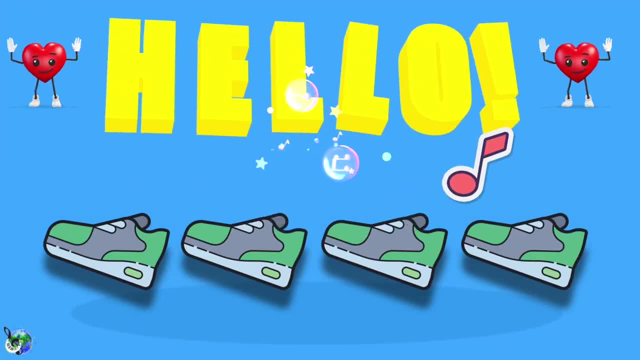 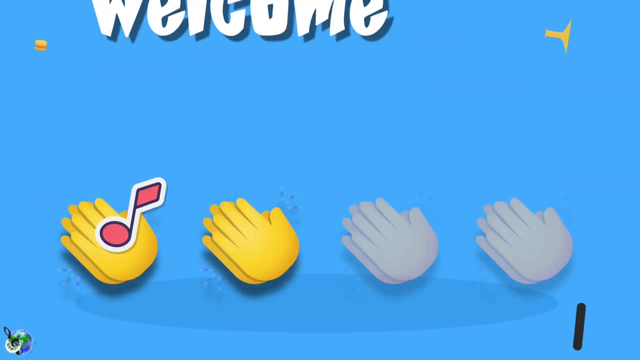 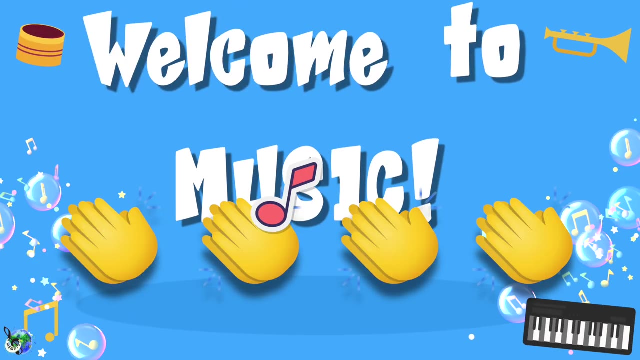 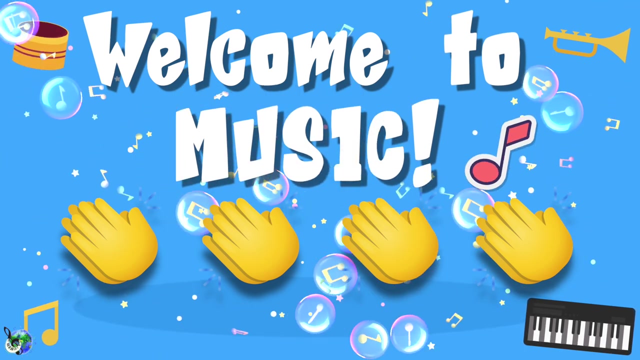 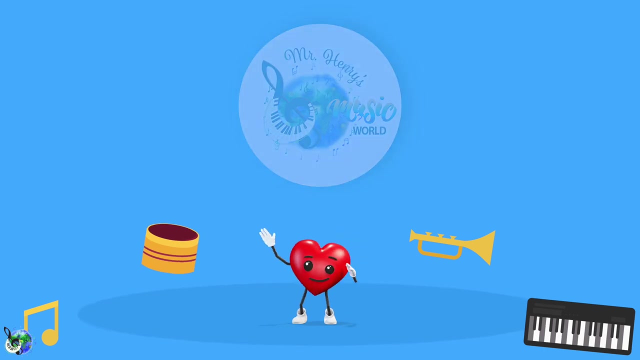 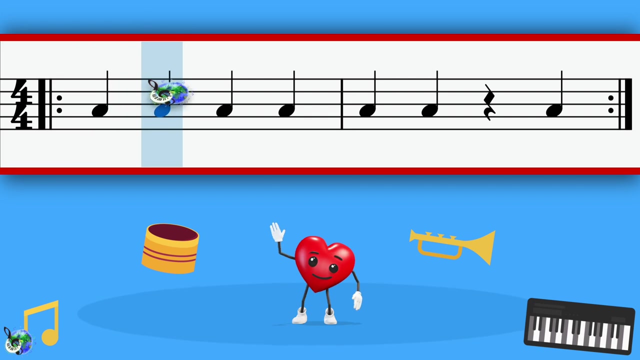 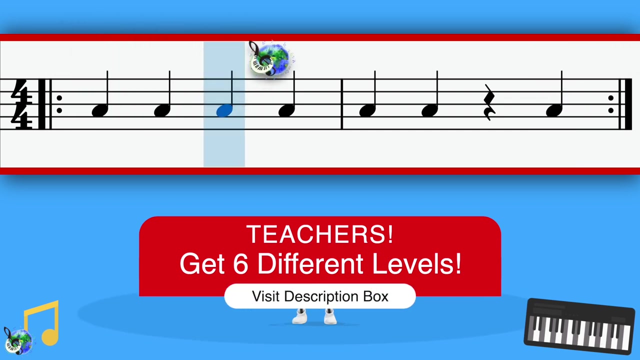 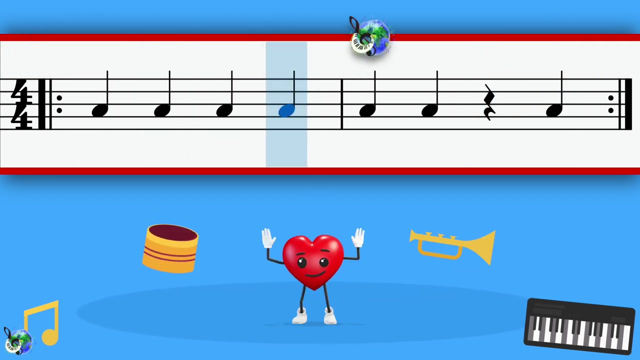 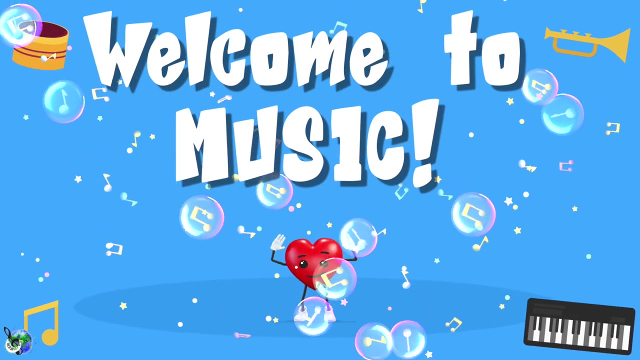 and grooving to music town. Hello welcome to music. Oh yeah, it's time to get your instruments or clapping hands ready to perform the rhythms coming your way. Here we go. Hello welcome to music. Hello welcome to music.